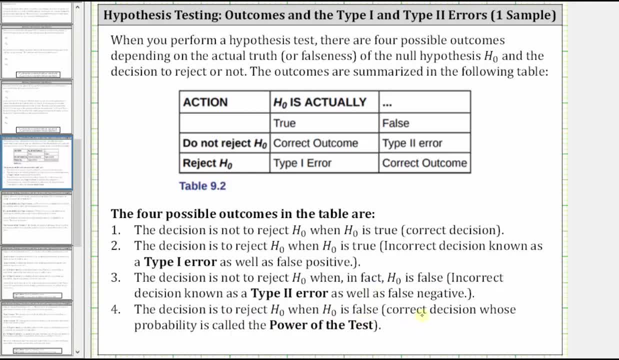 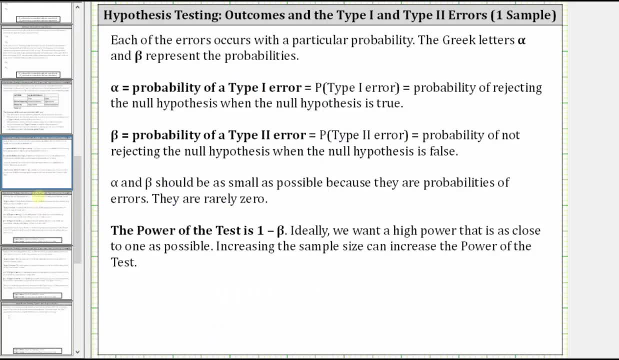 when the null hypothesis is false. This is a correct decision, whose probability is called the power of the test. Each of the errors occurs with a particular probability. The Greek letters alpha and beta represent the probabilities. Alpha is equal to the probability of a type one error. 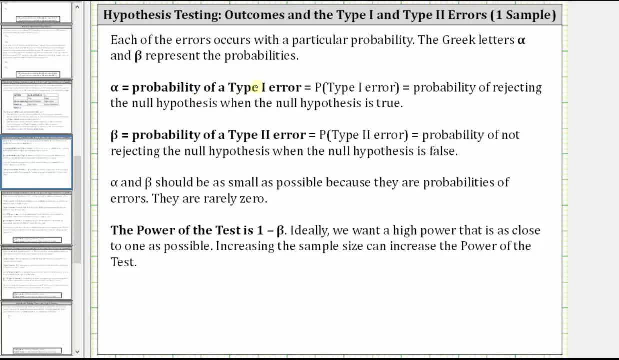 which is the probability of rejecting the null hypothesis when the null hypothesis is true. Beta is equal to the probability of a type two error, which is the probability of not rejecting the null hypothesis when the null hypothesis is false. Alpha and beta should be as small as possible. 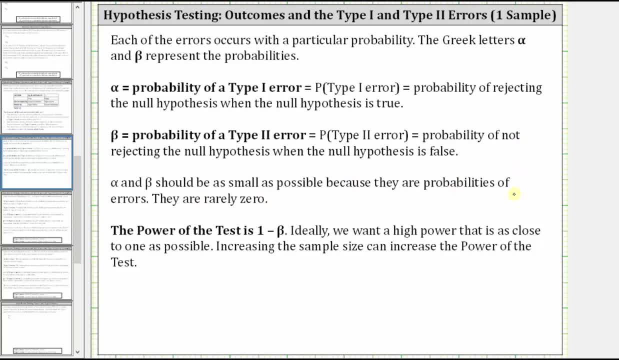 because they are probabilities of errors. However, they are rarely zero. The power of the test is one minus beta, where beta is the probability of a type two error. Ideally, we want a high power that is as close to one as possible. 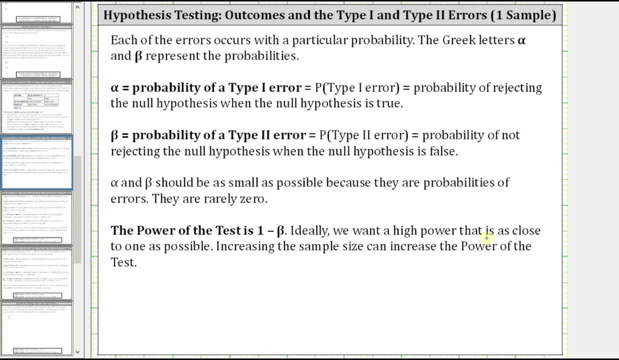 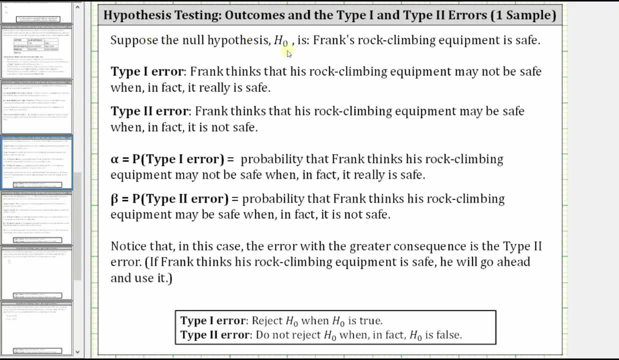 Increasing the sample size can increase the probability. This can increase the power of the test. And now let's take a look at some examples. For the first example, we will suppose the null hypothesis is Frank's rock climbing equipment is safe. So again, the type one error would be: 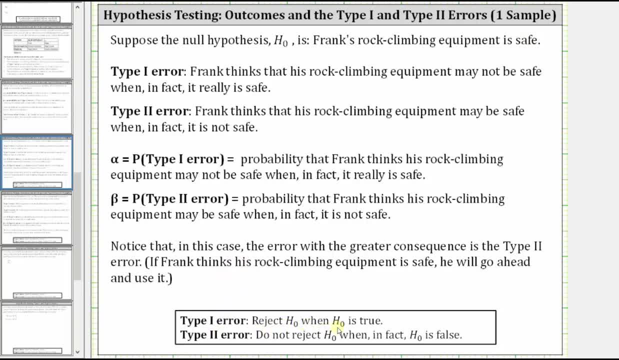 the decision to reject the null hypothesis when the null hypothesis is true. So for this situation, the type one error would be: Frank thinks that his rock climbing equipment may not be safe when in fact it really is safe. Again, the decision to reject the null hypothesis. 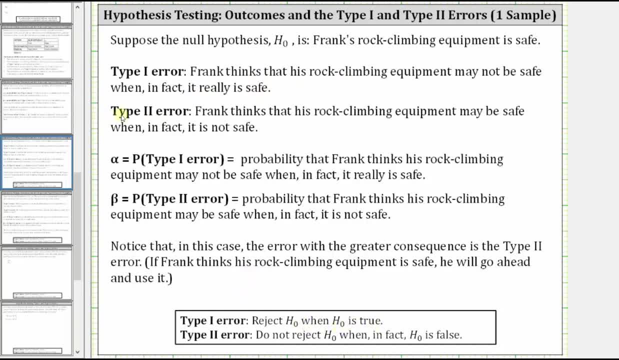 when the null hypothesis is true. And now for the type two error, which is a decision to not reject the null hypothesis when in fact the null hypothesis is false. In this situation, the type two error would be: Frank thinks that his rock climbing equipment may be safe. 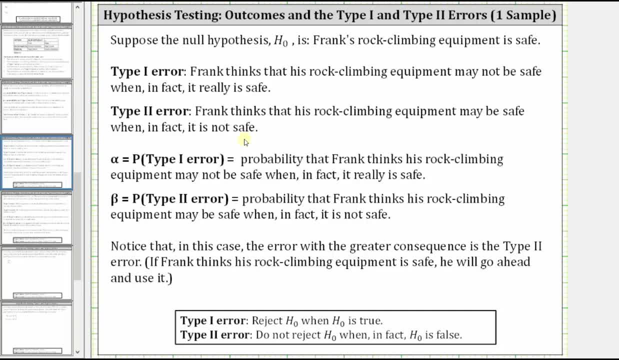 when in fact it is not safe. Again, this is because we are not rejecting the null hypothesis when in fact the null hypothesis is false. From here it follows that alpha, the probability of the type one error, is the probability that Frank thinks his rock climbing equipment may not be safe. 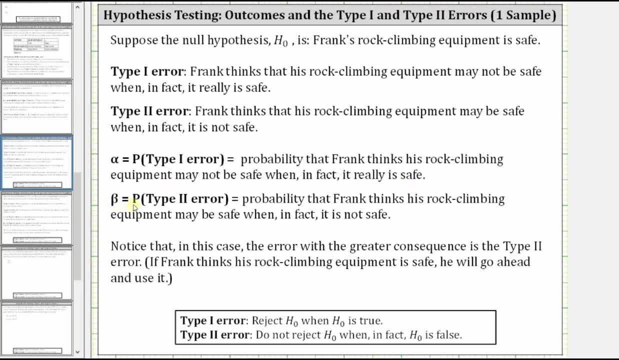 when in fact it really is safe. And beta is the probability of the type two error, which is the probability that Frank thinks his rock climbing equipment may be safe when in fact it is not Notice. in this case, the error with a greater consequence.